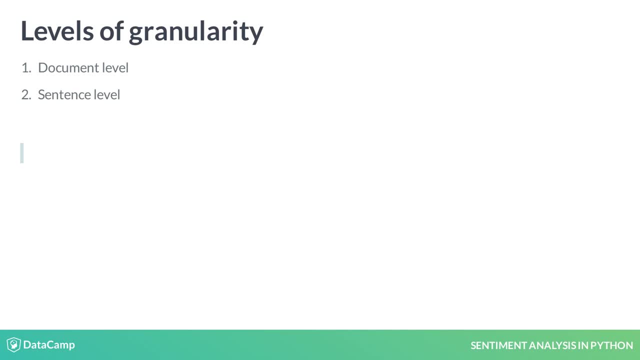 Second is the sentence level. This refers to determining whether the opinion expressed in each sentence is positive, negative or neutral. The last level of granularity is the aspect level. The aspect refers to expressing opinions about different features of a product. Imagine a sentence such as the camera in this phone is pretty good, but the battery life is disappointing. 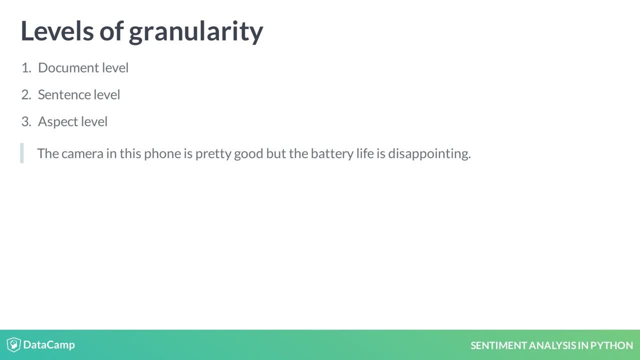 It expresses both positive and negative opinions, And we might want to be able to say which features of the product clients like and which they don't. The algorithms used for sentiment analysis could be split into two main categories. The first is rule- or lexicon-based. 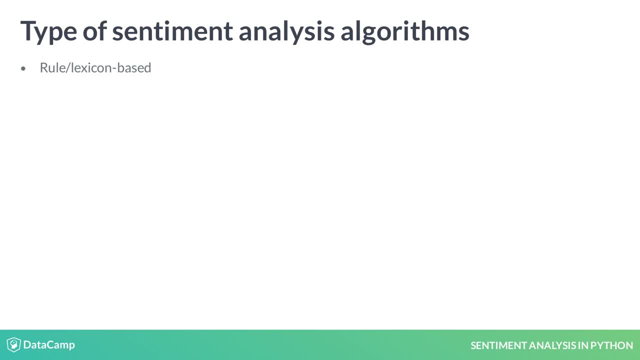 Such methods most commonly have a predefined list of words with a valence score. For example, nice could be plus two, good plus one, terrible minus three, etc. The algorithm then matches the words from the lexicon to the words in the text and either sums or averages the scores in some way. 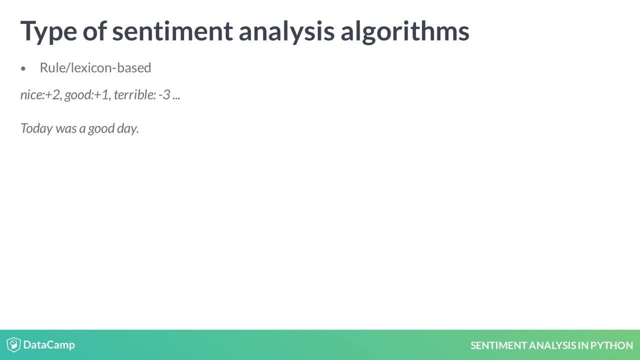 As an example, let's take the sentence: today was a good day. Each word gets a score and to get the total valence we sum the words. In this case, we have a positive sentence. A second category is automated systems. 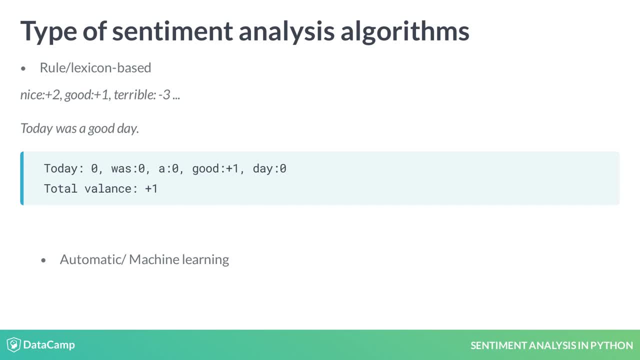 which are based on machine learning. This is going to be our focus in this course. The task is usually modeled as a classification problem where, using some historical data with known sentiment, we need to predict the sentiment of a new piece of text. We can calculate the valence score of a text using Python's text blob library. 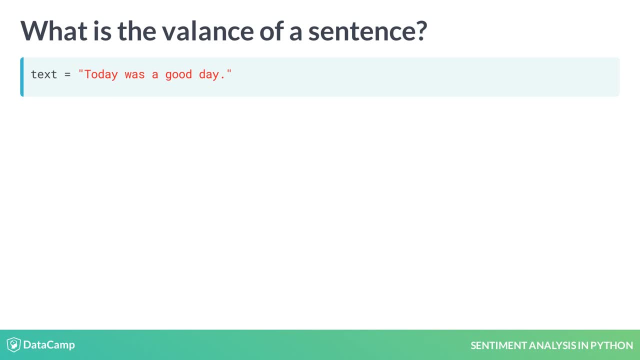 We continue working with our today was a good day string. We import the text blob function from the text blob package and apply it to our string. A text blob object is like a Python string which has obtained some natural language processing skills. We can call different properties of the text blob object.